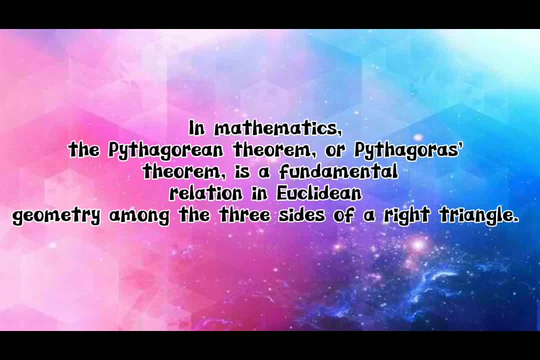 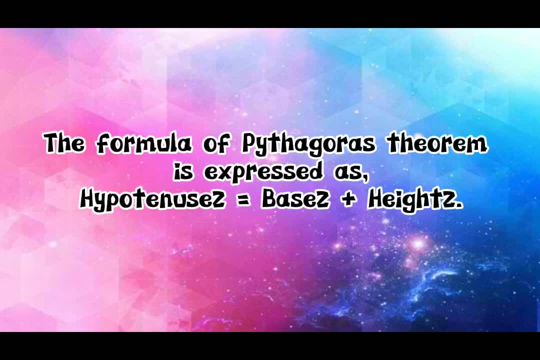 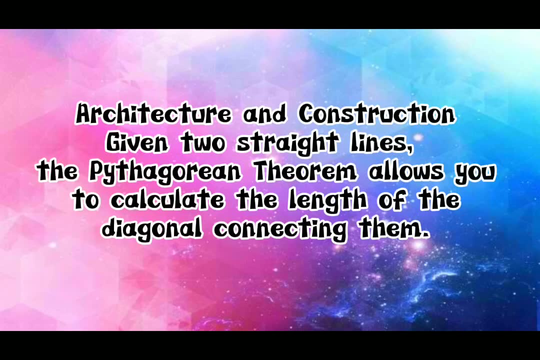 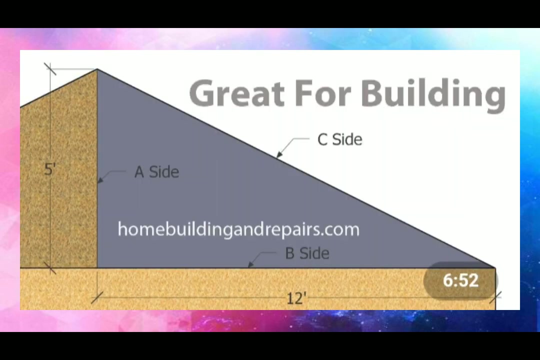 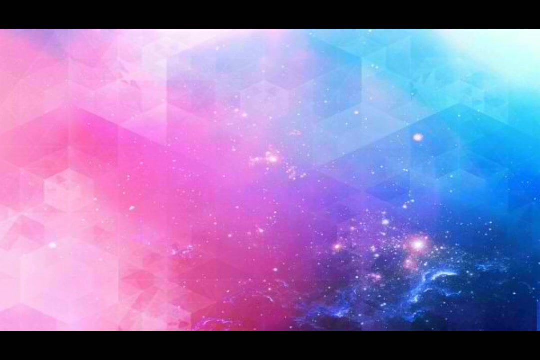 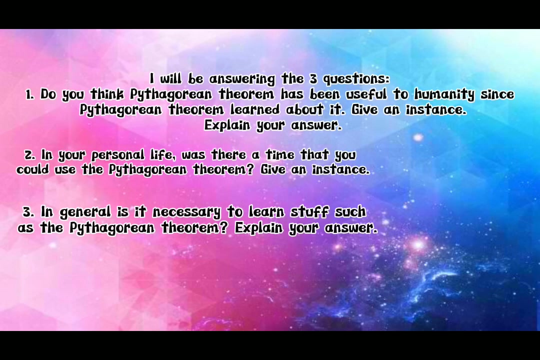 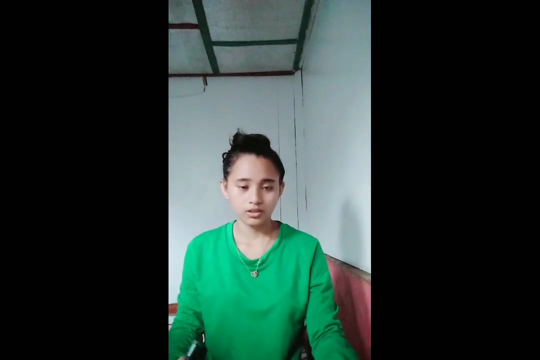 Introduction: Hi, so our teacher gave us questions, some questions that we must go in to answer. So the first question is: do you think Pythagorean Theorem has been useful to humanity since it was invented? If so, what is the most important use of Pythagorean Theorem? Give an instance. 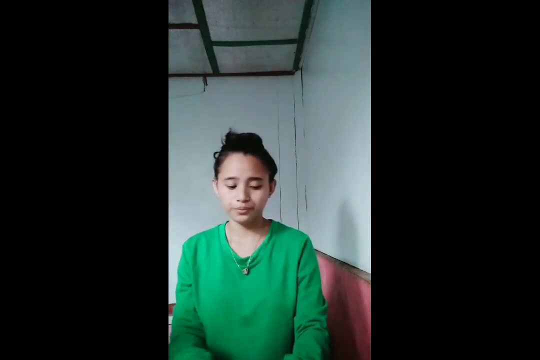 explanation to your answer. So my answer is: I will just go in to read the important use of Pythagorean Theorem. So this is: Pythagorean Theorem was discovered, lead to the Greek to prove the existence of numbers that could not be expressed as rational numbers. 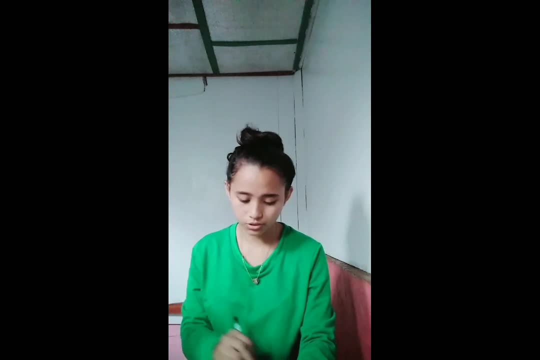 So taking two short sides of a right triangle to be one and one, we are lead to a hypotenuse or length, which is not a rational number. So Pythagorean Theorem is useful for two-dimensional navigation. you can use it in two length of five shortest distance. painting wall painter. 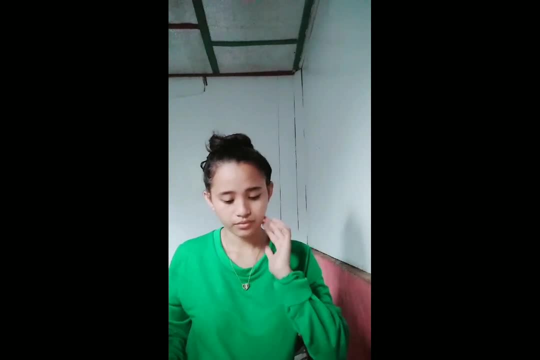 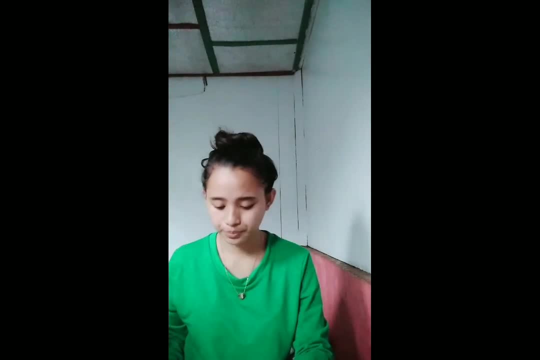 so helpful. example of being helpful to this is the painter. So a painter uses- what do you call this? A ladder to paint on a wall. So the painter must be adjust the ladder so that he can paint on a wall that he needs. 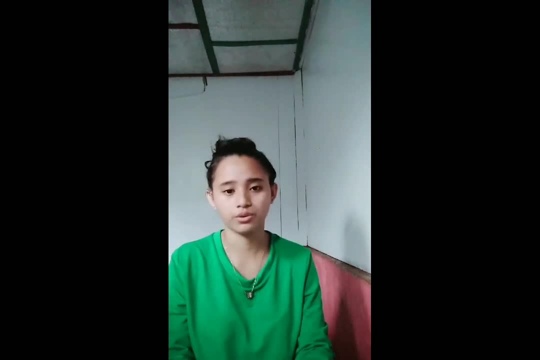 to be painted. He or she needs to be painted. So it example for it it was the some construction works or buildings. this is the example of buildings, a great uh architecture. so some of part of architecture classes needed to know about that, but pythagorean theorem, so that they will know how to angle they, their projects, how they were going. 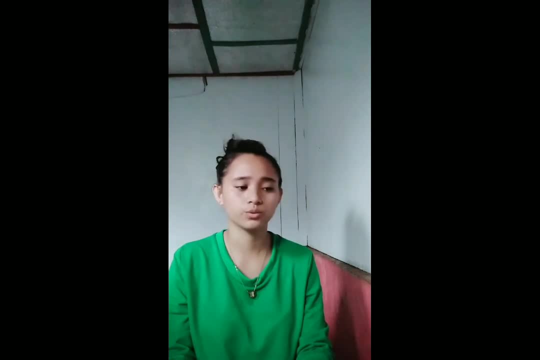 to adjust some movement, to adjust some angle so that it will not be going to look like so, so what? you call this so disturbing to others? so in so? second, the question is: in your personal life, were there, was there a time that you could use the pythagorean theorem? 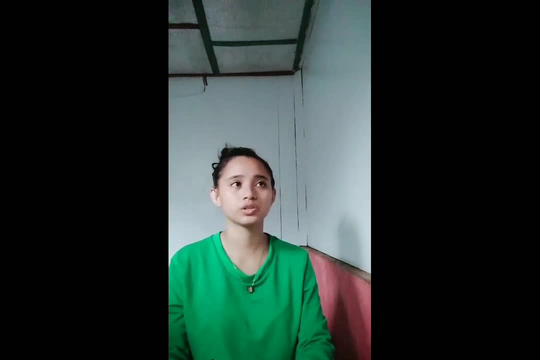 give an instance. so in my, In personal life, I am the first daughter of our family, so I'm also going to help my father to create some chairs, tables. So in creating it we need a measurement, we need to cut, we need to have to make an angle on how will we going to place the chair and the table so that it can fit to the room. 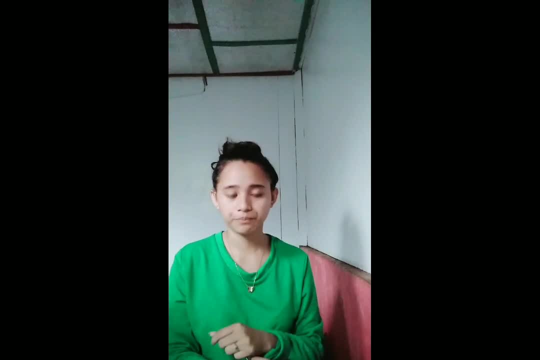 So the third question is: in general, is it necessary to learn stuff such as the fit Pythagorean theorem? explain your answer. So it is really necessary to know and learn about the Pythagorean theorem because it is a basic. I think it is a basic theorem where all people can use it, like making chairs or any tables, or the creating of building with the use of architecture. 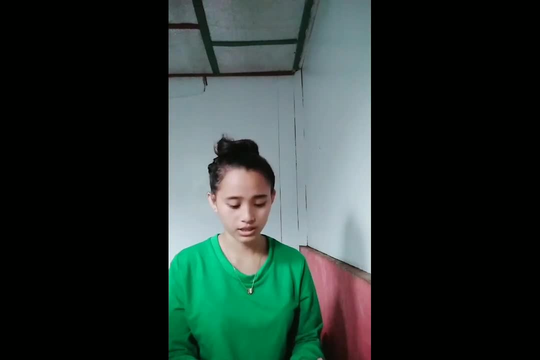 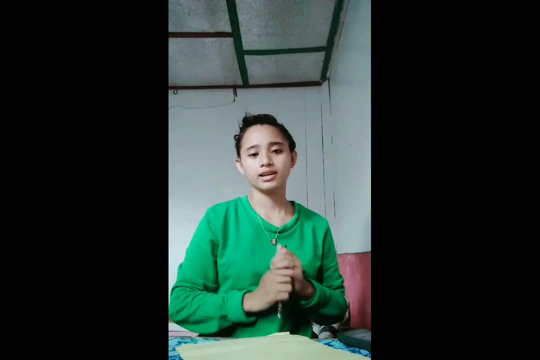 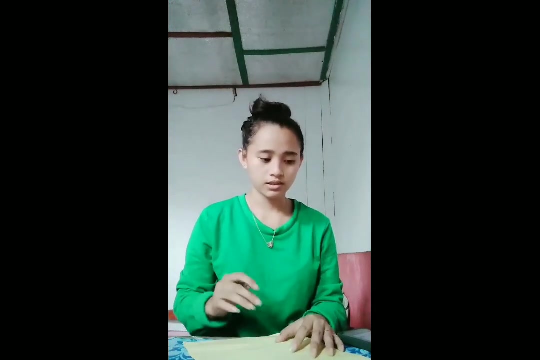 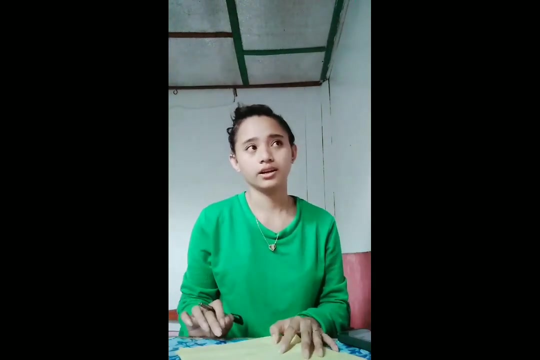 Pythagorean theorem is so helpful and must be learned, So it is really necessary to learn by everyone. maybe not everyone will going to learn that, but it is necessary to learn. Thank you, Hi guys, welcome to my video. This will be the last part of the video and in this situation I'm going to solve a Pythagorean theorem where I just search a equation in it. 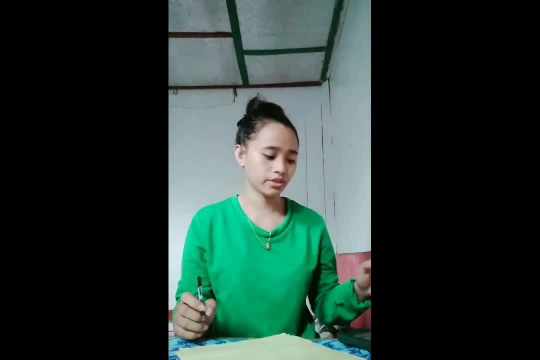 And I'm going to solve a Pythagorean theorem And I'm going to solve a Pythagorean theorem where I just search a Pythagorean theorem, where I just search a Pythagorean theorem, I was. I will be the one who will going to answer this. 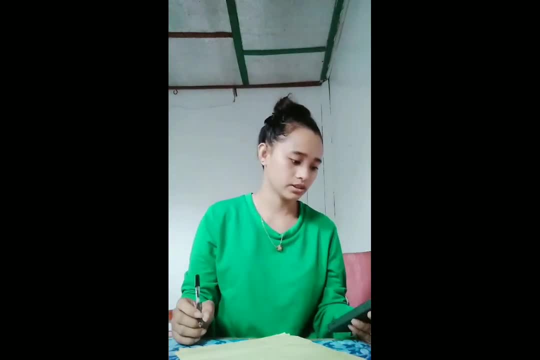 So the chosen one that I will be answering is: a ladder 13 meters long is placed in the ground in such a way that it touches the top of the vertical wall 12 meters high. Find the distance of the foot and of the ladder from the bottom of the wall. 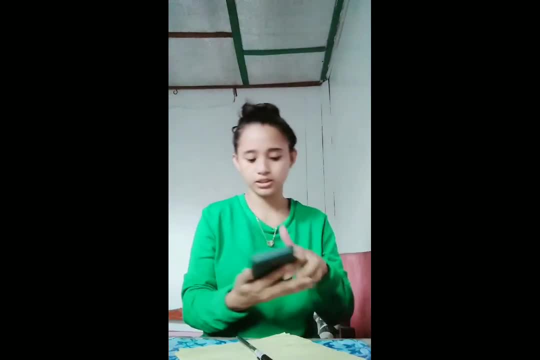 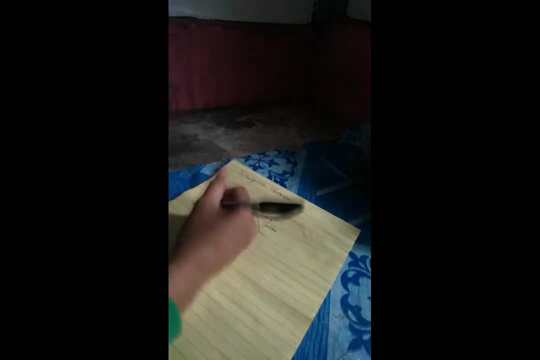 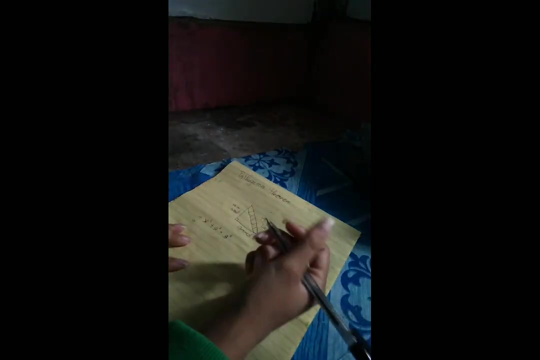 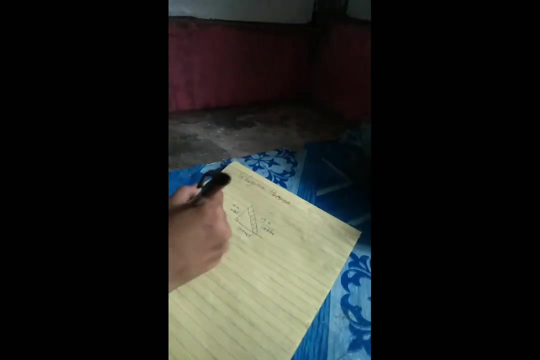 So this is will be the picture of the ladder and the ground, So that will be the equation that I'm going to answer. So this is really the situation that we are going to go to: Plus 10, vertices 13, plus 12.. 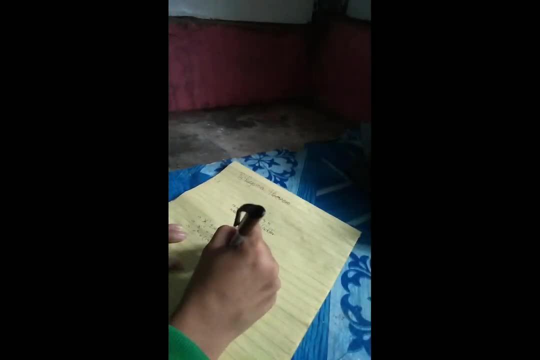 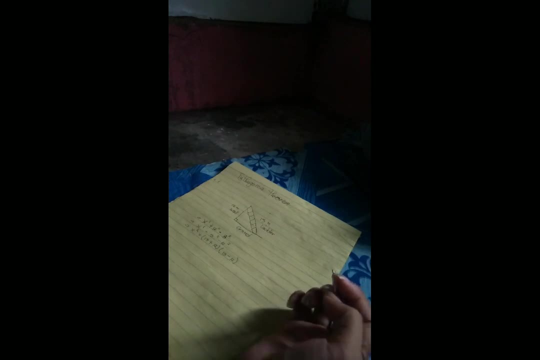 Yeah, okay, So 13. D minus 12. No, Global V: This is the old V baby. So then I'm saying this is initial plus, This one is initial Zero. Oh no, Oh no.